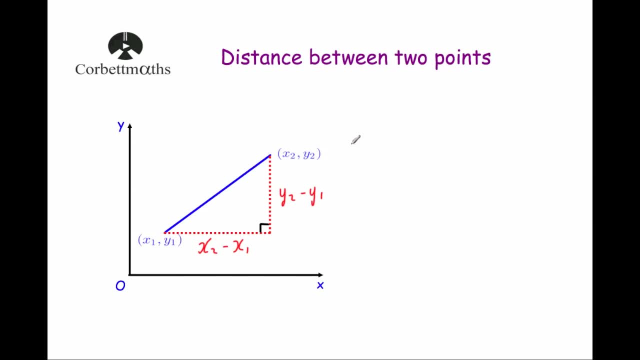 And now we're going to use Pythagoras' theorem to work out the length of the hypotenuse. So Pythagoras' theorem is a squared plus b squared. Now let's call the length of the hypotenuse d, so that's the distance between the two points. 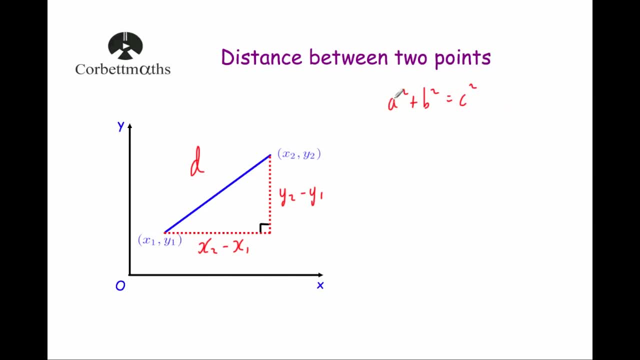 and let's substitute these into the formula. So a squared, that's one of the shorter sides, so let's call it this first one. So that's going to be x2 minus x1 squared, plus the other shorter side, that's this one. so it's going to be y2 minus y1 squared and that's equal. 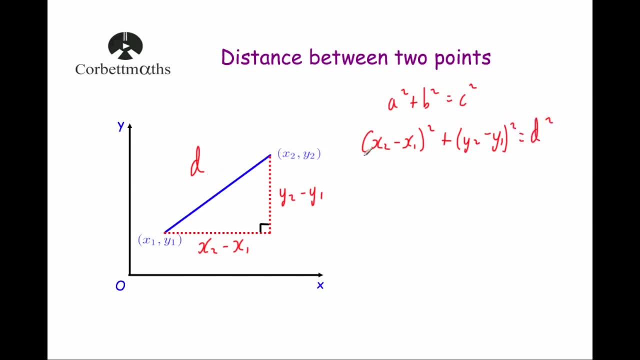 to the hypotenuse squared and that's going to be d squared. Now we don't want to know d squared, we want to know d. so we're going to take the square root both sides of this equation. so it's going to give us the square root. this is: 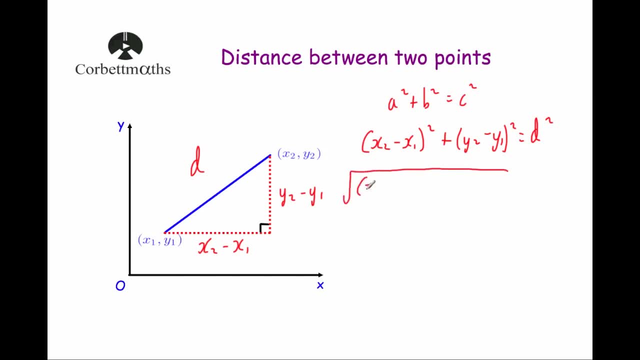 going to be a big square root sign going right over the top and we've got x2 minus x1 squared plus y2 minus y1 squared, and that's equal to d. and that's it. So this is the formula to work out the distance between two points. Let's have a look at it typed out. so we've got the distance d. 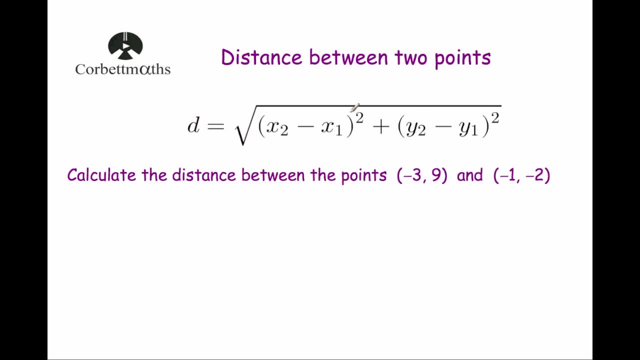 is equal to the square root of x2 minus x1 squared, plus y2 minus y1 squared, and that's it. Now, in terms of labeling the points, we can call either one of them x1 y1 and x2 y2.. I tend 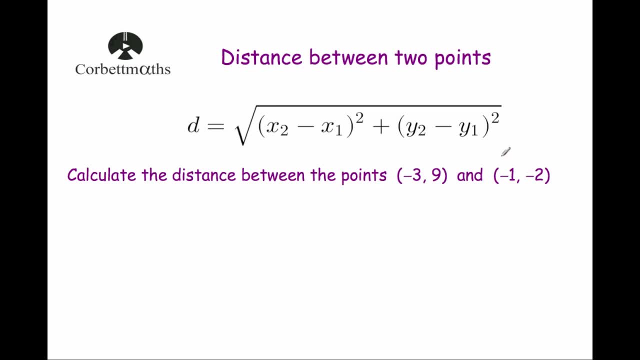 to just call the first one that I see, x1, y1 and the second one, x2, y2.. It doesn't matter, because we're going to be squaring them. if we were had to have a negative instead of a positive when we square, we're just going to get positive values anyway. So let's label the points. there's our. 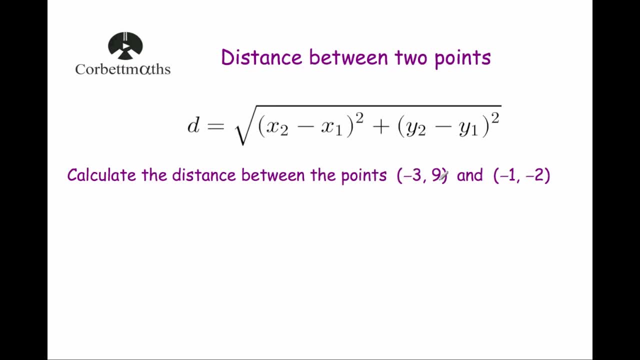 first question. it says: calculate the distance between the points negative three, nine and negative one, negative two. So I'm going to call my first coordinate x1, y1 and my second coordinate x2, y2.. So let's substitute these points into our formula. so we've got: d is equal to the. 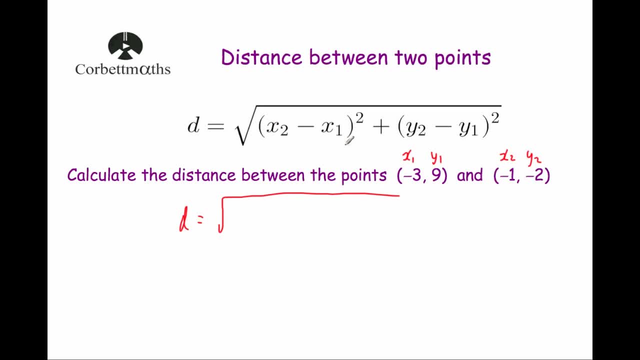 square root of, and we've got x2 minus x1, so x2 is equal to minus one and we're going to be subtracting x1. so that's negative three. so we'll be subtracting negative three, squared then plus, and then we've got y2, so y2 is equal to negative two and we're going to be subtracting y1. so 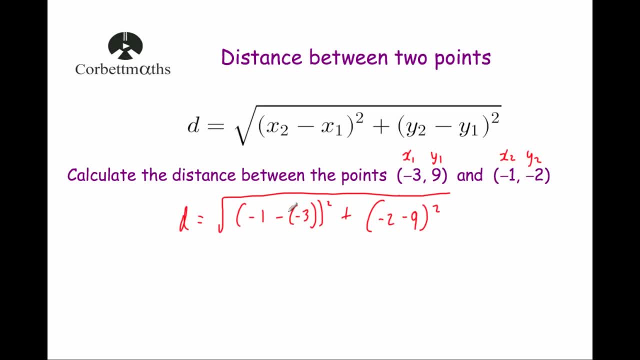 subtract nine squared. I'm just going to carry on the square root of it. Let's work out the brackets. so d is equal to the square root of. so minus one, minus minus three. so it's going to be minus one plus three. that's going to be two squared plus, and then our other bracket. 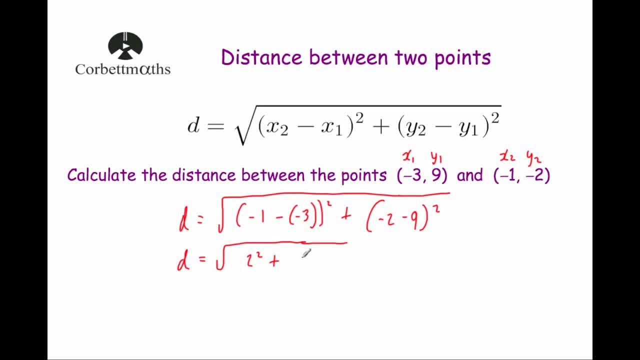 we've got minus two. take away nine. now, minus two, take away nine is negative eleven or minus eleven squared. so d is equal to the square root of and we're going to square these. so two squared is equal to four and minus eleven squared. well, minus eleven times minus eleven is 121, so it's plus 121.. 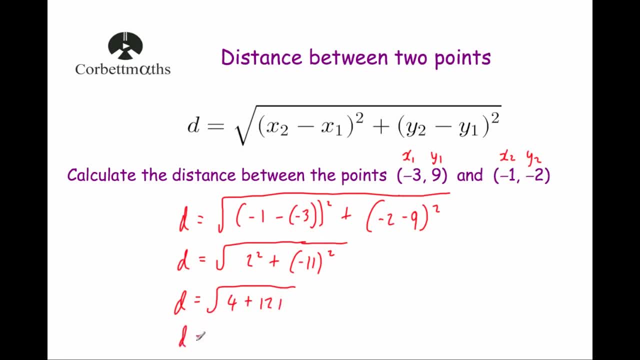 Now we're going to work out four plus 121, so d is equal to the square root of 125, and now we just need the square root that to get d, the distance between the two points. so when we do that, the square root of 125 that could be five root five, or it could be if you want to write it as a decimal. 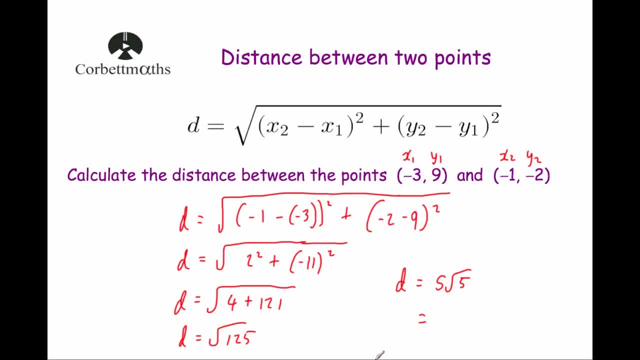 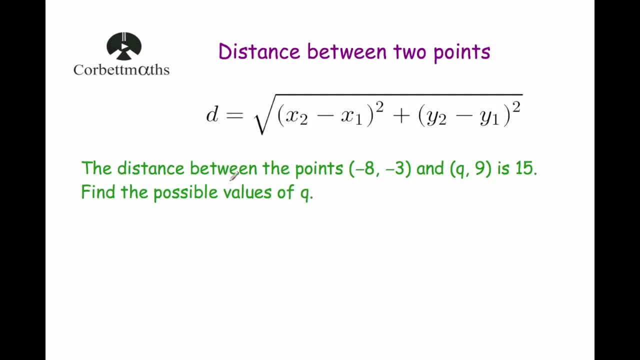 the square root of 125 is equal to 11.18, and that's it. Okay. so let's have a look at our second example. so our second example says the distance between the points minus eight, minus three and q nine is equal to 15.. So then this question: we've been given the distance between 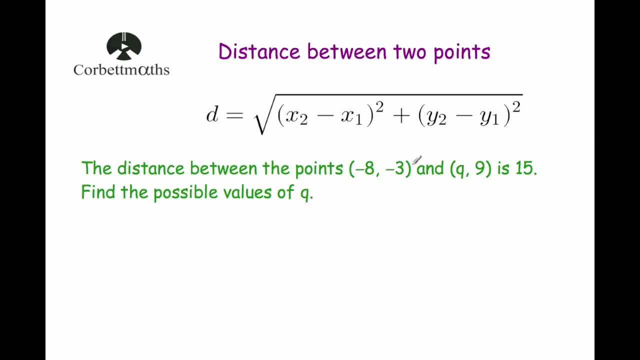 the points. we've been asked to work out the possible values for q. so, first of all, what we're going to do is we're going to label the points x1, y1, x2, y2 and d, I suppose. so we're going to get d. 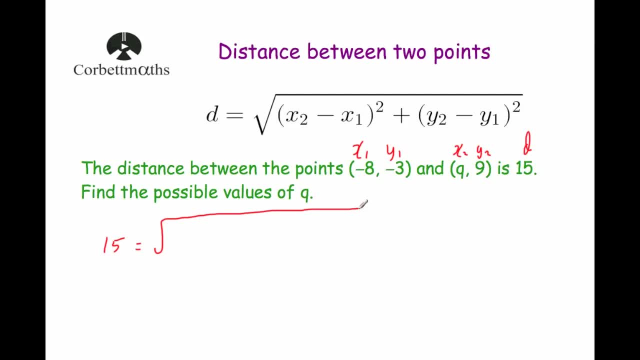 is 15, equals the square root of brackets y2, so it's going to be equal, or x2, so x2 is equal to q subtract x1, which is minus two minus eight. close brackets squared plus. and then the second bracket, y2, that's going to be nine minus. 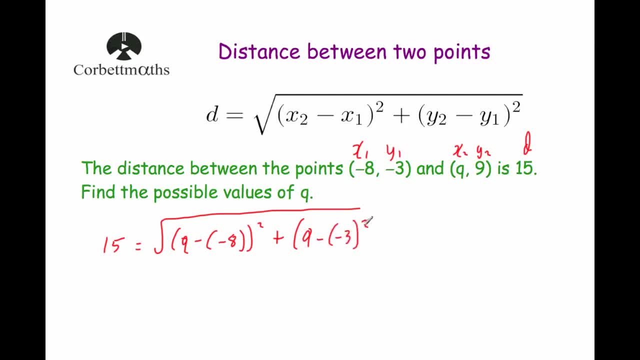 y1, that's going to be equal to minus three close brackets squared. and now let's simplify these brackets. so we're going to get: 15 is equal to the square root of, and we've got q minus minus eight. so it's going to be q plus eight squared. and the second bracket we're going to have nine. 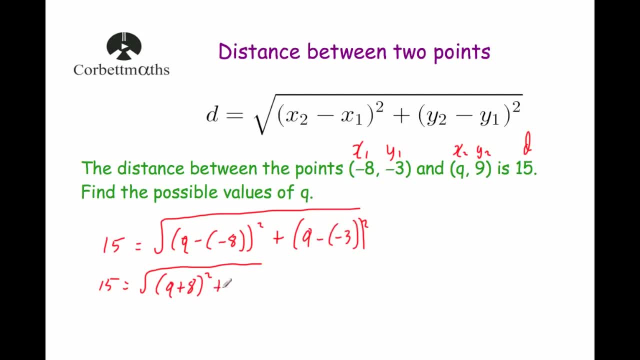 minus minus three, so it's going to be nine plus three, which is twelve. so plus twelve squared- So we're going to have 15- is equal to the square root of q plus eight squared plus 144.. Now I want to get rid of the square root sign. so what I'm going to do is I'm going to square both. 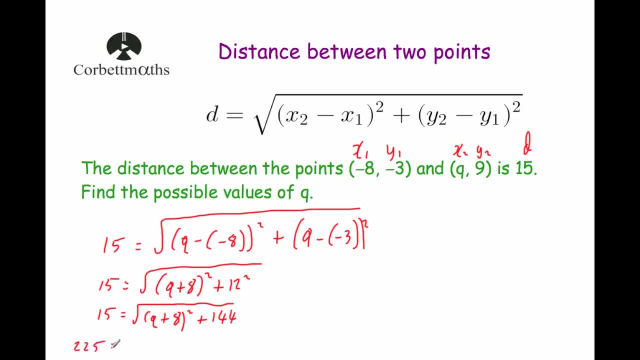 sides of the equation, and when I do that I get 225 equals, and squaring the right hand side will just get rid of the square root symbol. so it's going to be q plus eight, squared plus 144.. Now we want to find q, so let's subtract 144 from both sides of the equation. 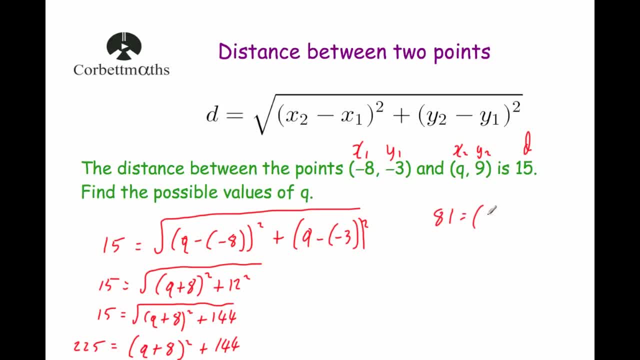 So that'll leave us with 81 equals q plus eight squared. Now we've got q plus eight squared, so we're going to square root both sides of the equation. but just remember that a positive times a positive can be 81, but a negative times a negative can. 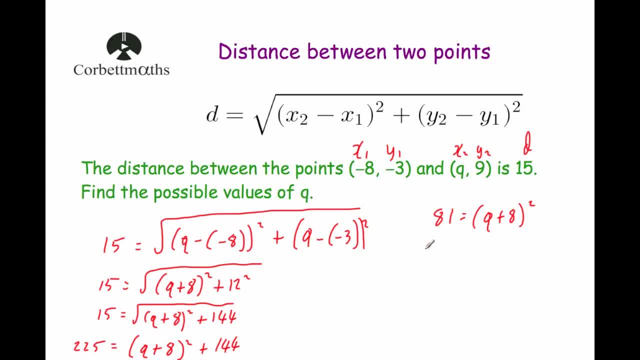 also be 81, so we're going to square both sides. but remember we're going to have the positive and negative solution. so square square is in. 81 will be nine, so it's going to be positive or negative. nine is equal to q plus eight, So we want to find q on its own. so we're going. 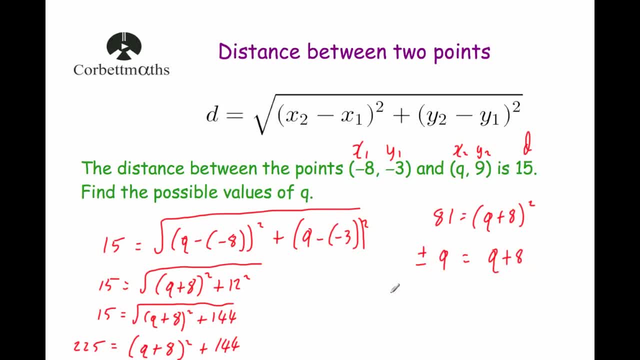 to get eight from both sides of the equation. so I'm going to subtract here from both sides and I'm going to put the eight at the front here. so minus eight plus or minus nine equals q, and when I do I get minus eight plus nine, so it's going to be equal to one. so q can be equal to one or q can. 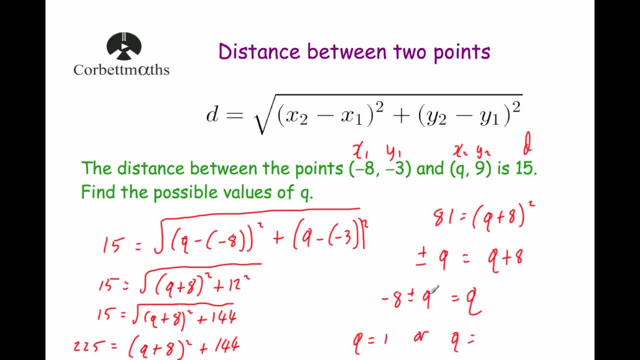 be equal to minus eight subtract nine, and minus eight subtract nine would be minus 17.. There are two solutions, so q could be equal to one or q could be equal to minus 17.. That's it, so the distance between two points can be worked out using the formula. 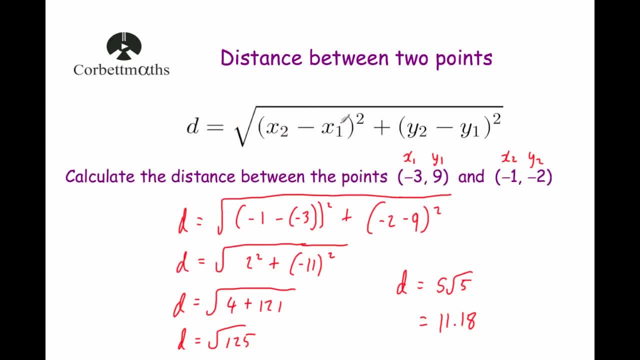 d equals the square root of x2 minus x1 squared, plus y2 minus y1 squared, and just remember that these two can actually be written either way around, so it could be y2 minus y1 squared plus x2 minus x1 squared. That's it.